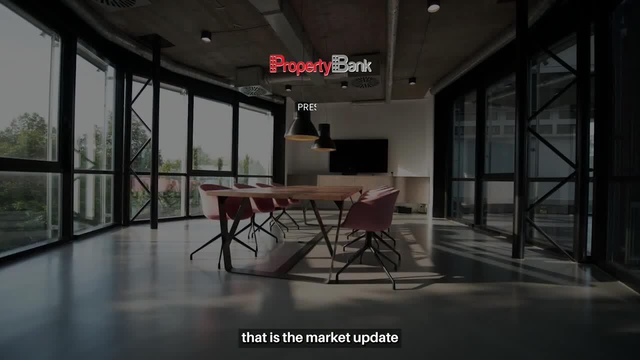 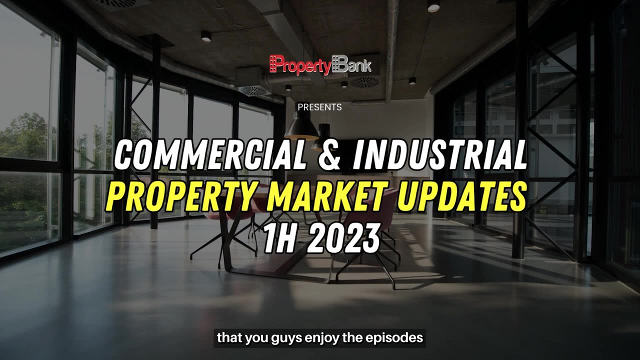 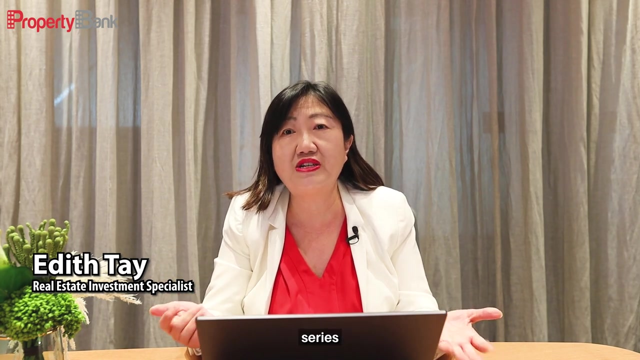 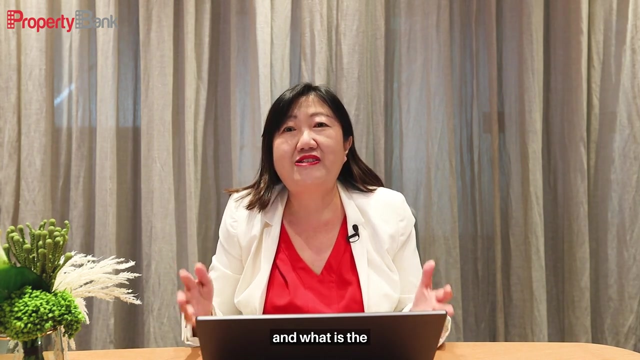 Welcome to yet another episode, that is, the market update of commercial and industrial properties and I'm really happy to see that you guys enjoy the episodes. What is different substantially from this YouTube series is that we give you the real source: what's transacted in the market and what is the upcoming pipeline. So first half have just gone in a glimpse of the 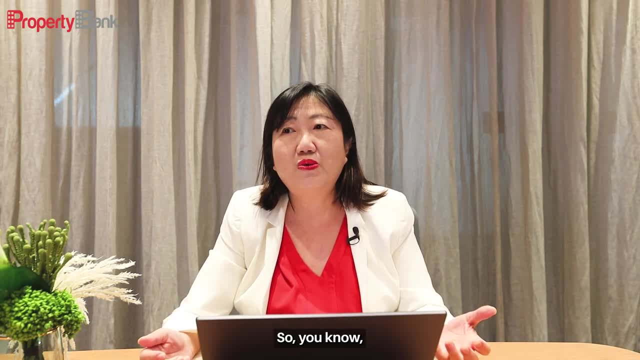 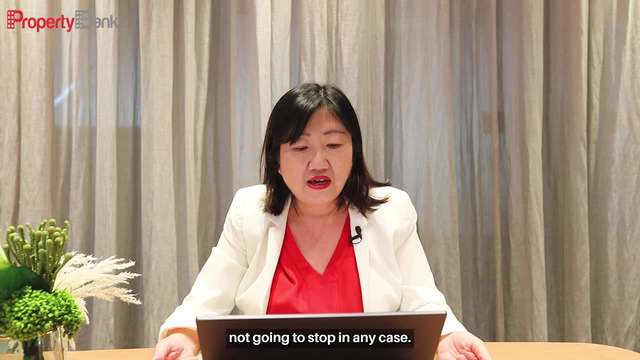 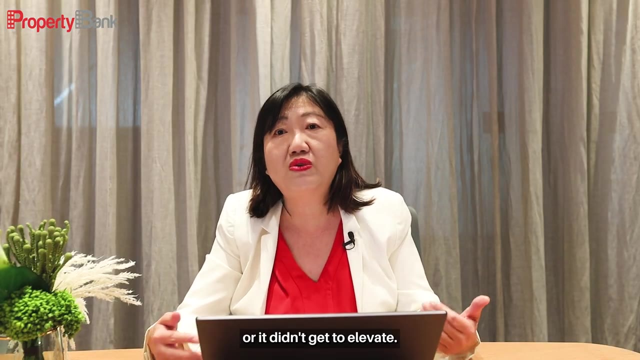 eyes and now we are into the third quarter. so you know, the war has continued and, seriously, it seems that it's not going to stop in any case, and the banking crisis doesn't really bother us too much, or it didn't get to elevate, so that's good news. Interest rate continues. 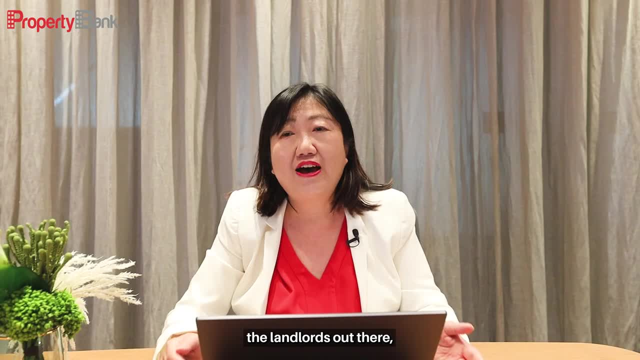 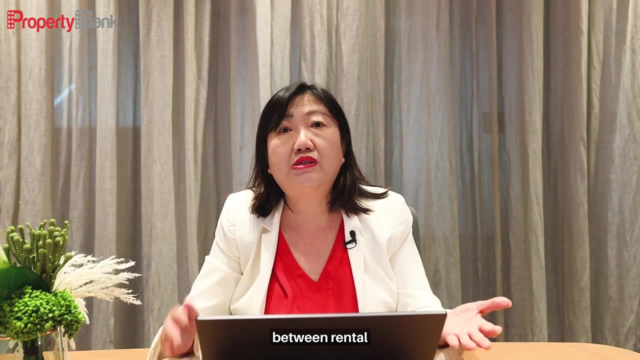 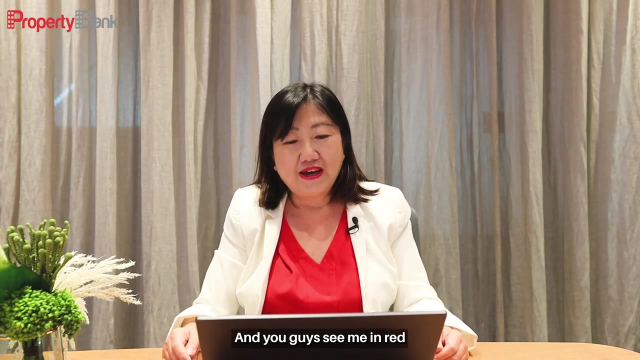 to be high. that means you, the landlords out there, have some opportunities to continue to retain your tenants. if they were to compare between rental and purchase, most likely because of the high interest rate, they will continue to be with you, and you guys see me in red and whites because today 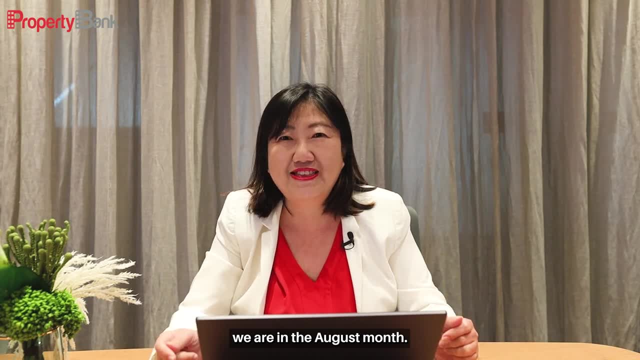 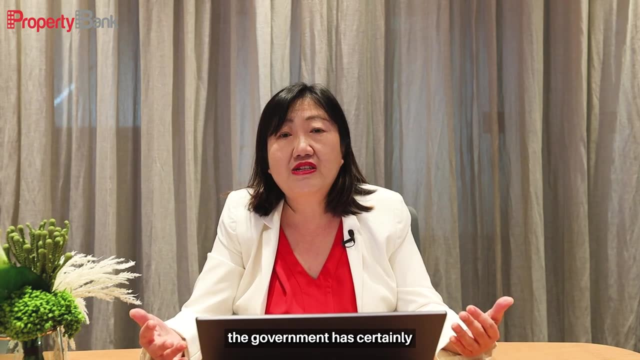 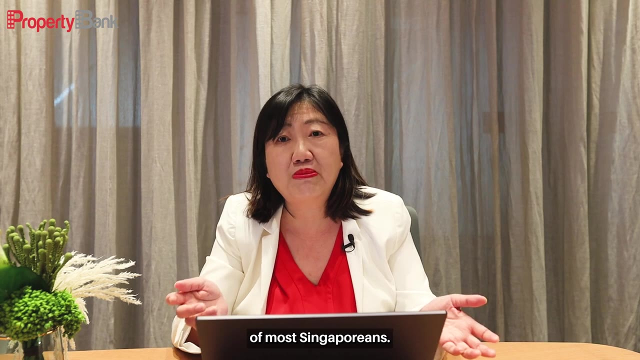 while we are filming this, we are in the August month. I want to stress upon I love Singapore and Singapore as an industrial town, a country. the government has certainly made sure that the residential properties are within the affordability of most Singaporeans And when it comes to commercial industrial properties, for the first time in the first 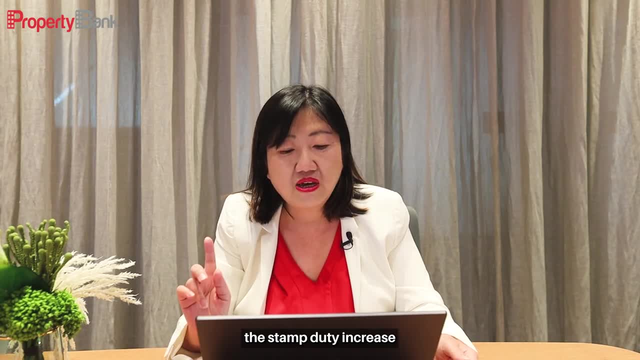 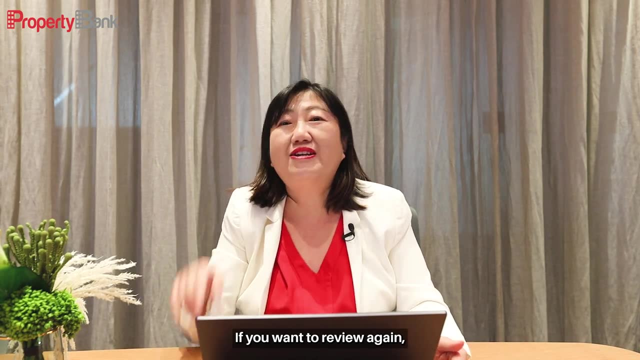 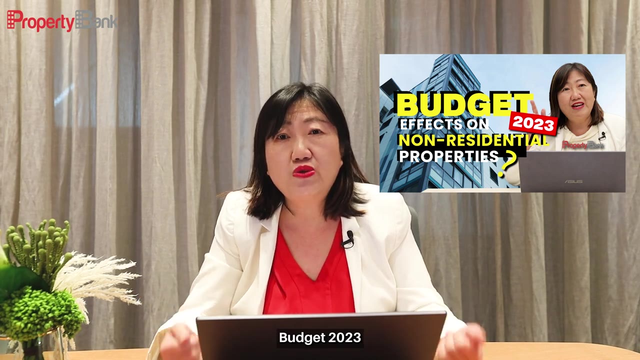 half of the year, you know that there's, for the first time, the stamp duty increase, which impacts on the non-residential properties. If you want to review again, click the button. watch the series that I have recorded for Budget 2023.. 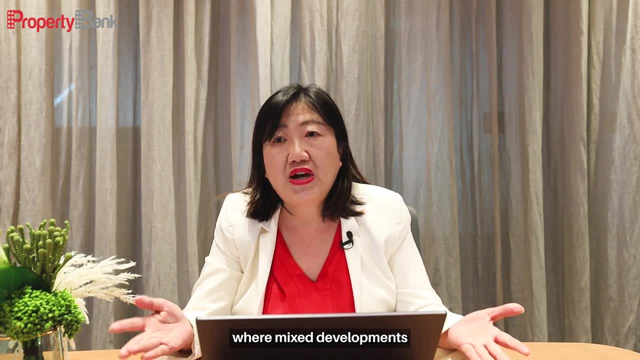 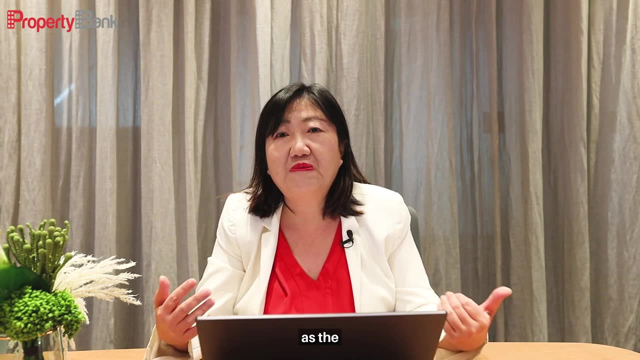 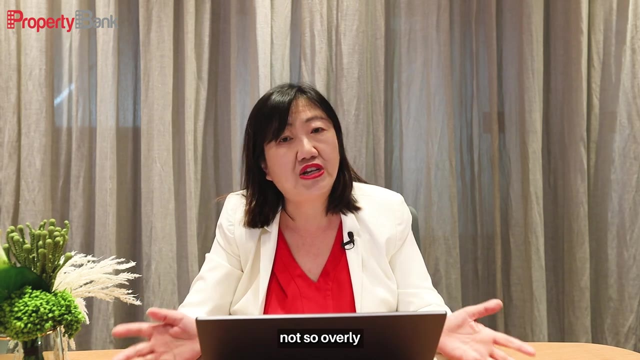 And of course in recently where mixed developments are concerned, for the commercial component is also kind of like treated as the residential tax portion, but most developers are actually not so overly concerned about it Because most of them actually don't care about it. 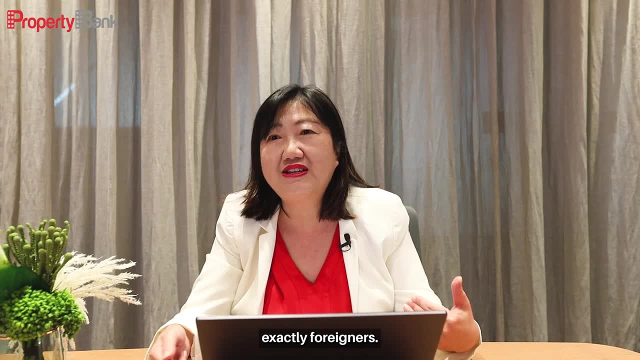 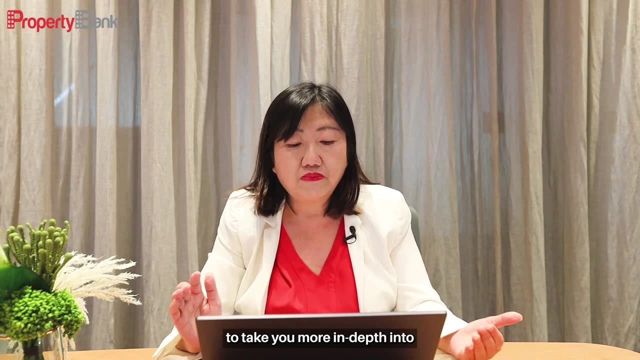 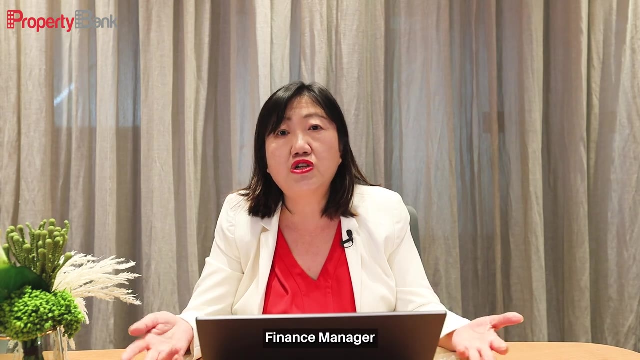 Most of them actually have local companies, so they are not exactly foreigners. So with that I would also like to take you more in-depth into if you are a business. in business, you are the HR and the finance manager looking at office relocation. what's? 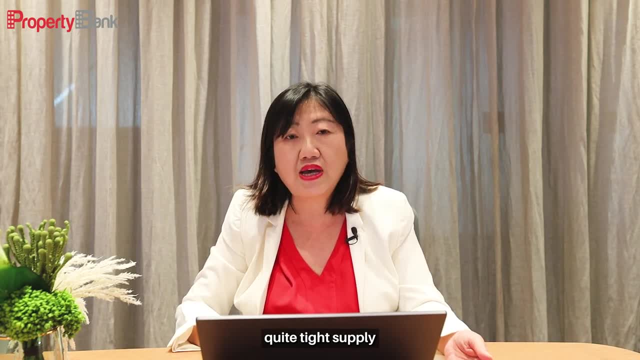 the current situation right now. In fact, we are facing quite tight supply in the market right now And also the amount of business that we have in the market right now is quite high, And also the amount of business that we have in the market right now is quite high. 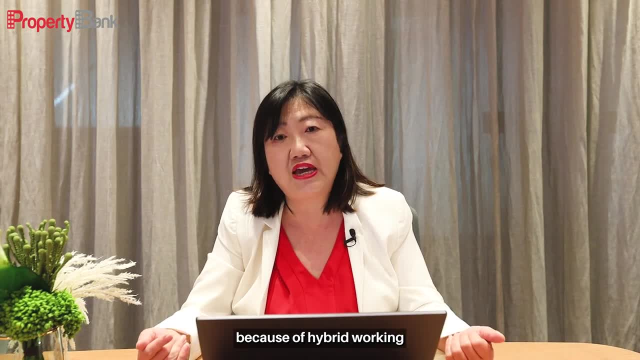 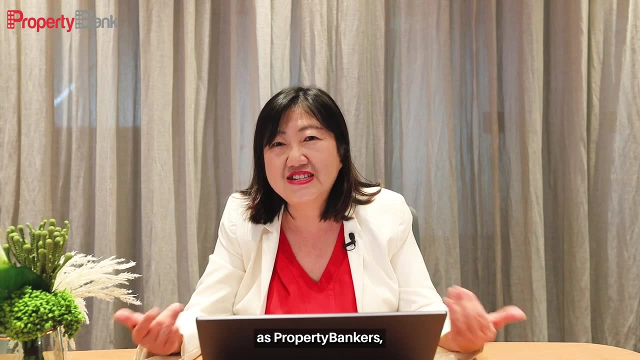 We work right with the benefits that we receive. So for us we have much left hand side because of hybrid working. you know, companies are sizeing their space And for us, as property bankers, we work with them to look at how to set up, to specify. 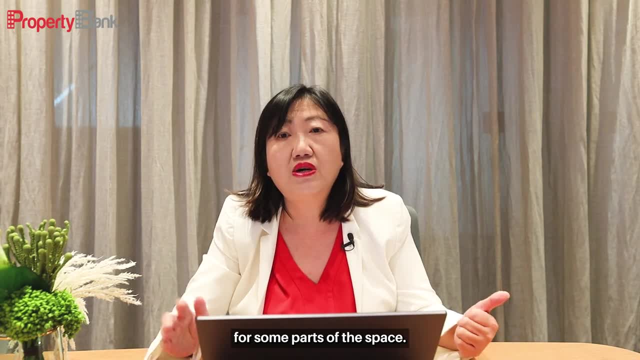 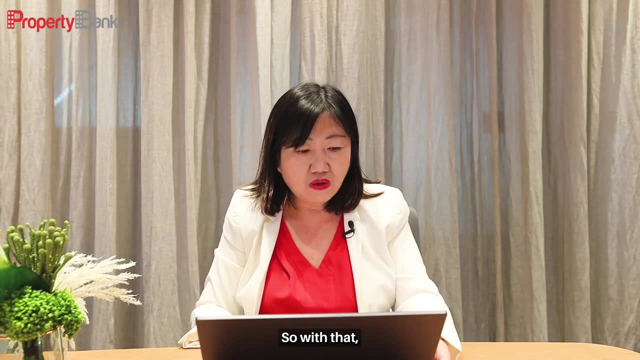 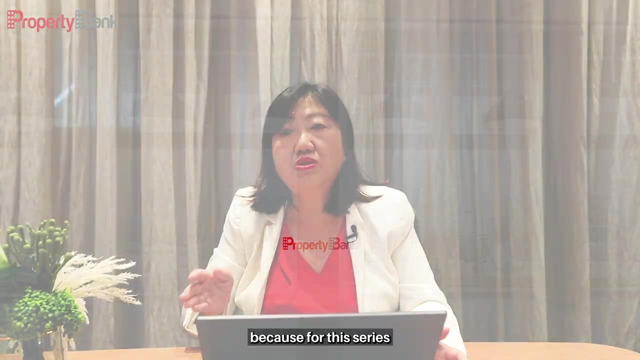 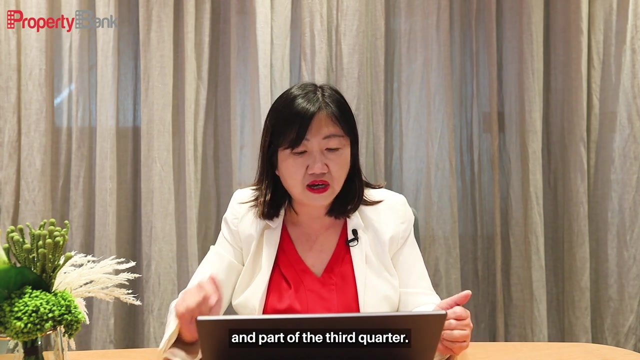 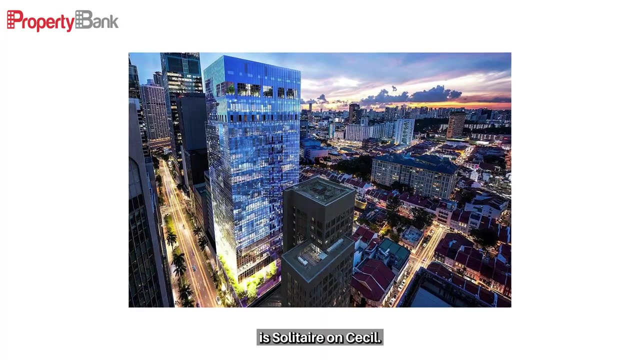 certain replacement tenants and then Ó help them that they want to relocate or rocket or renovate, because for this series we're talking about market and really what has happened in the market for the first half and a part of the third quarter. okay, so one of the very hot products or properties right now is Solitaire at 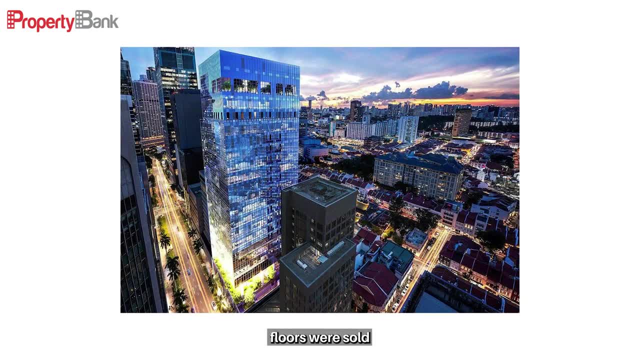 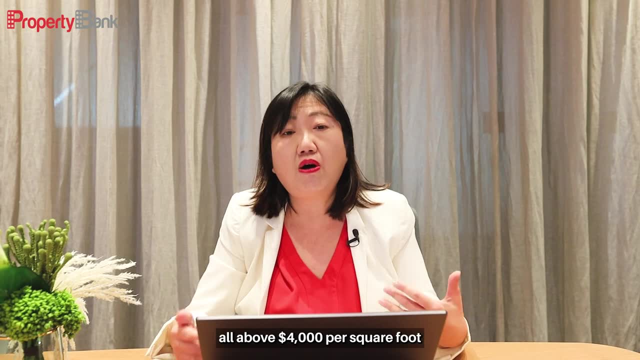 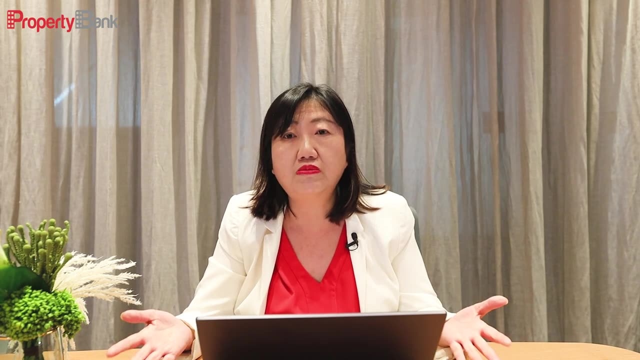 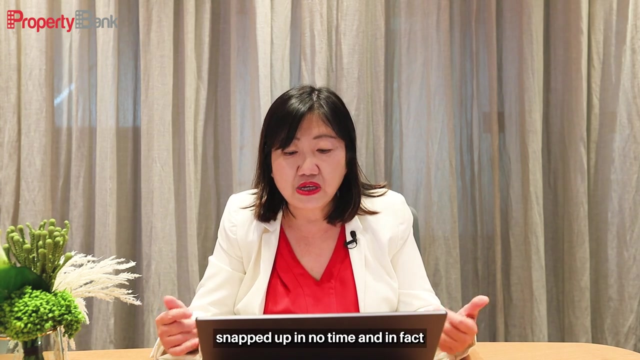 Cecil, can you imagine the total of 15 floors were sold within three months, fully sold and you know, in fact all above 4,000 per square foot, record breaking. but it is value that you know all these buyers are looking into free hold and really great a standard. so it's really step up in no time and in fact, 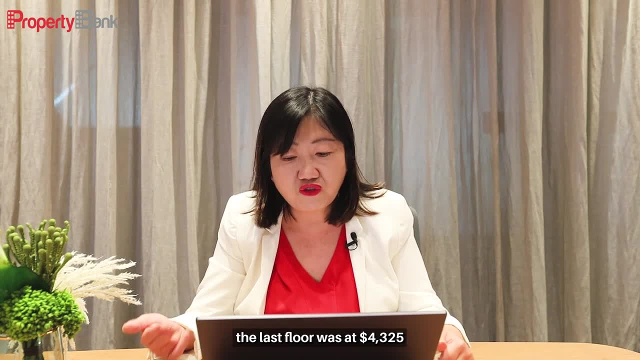 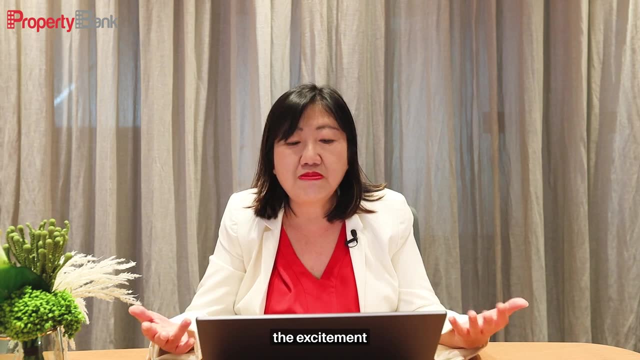 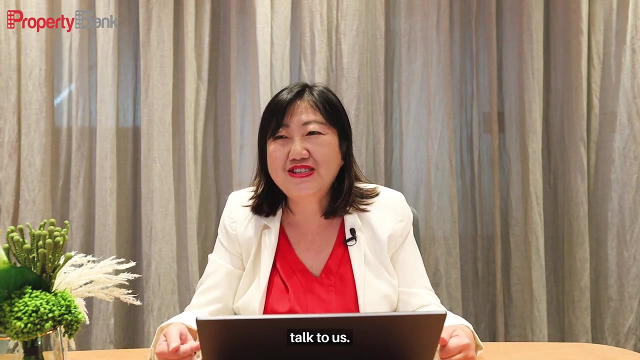 the last floor was at 4,325 per square foot, so you can see lots of news out there reporting about, you know the excitement of this property and really, for those of you who miss the boats, talk to us. we probably have others to offer you and you have Liberty House, okay, so at 92.2. 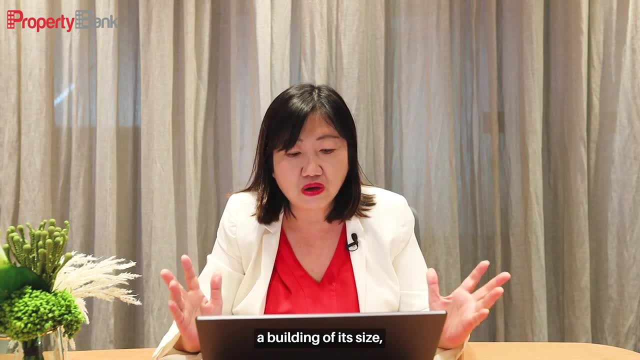 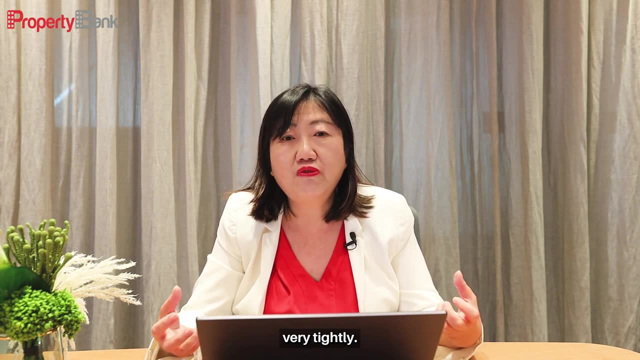 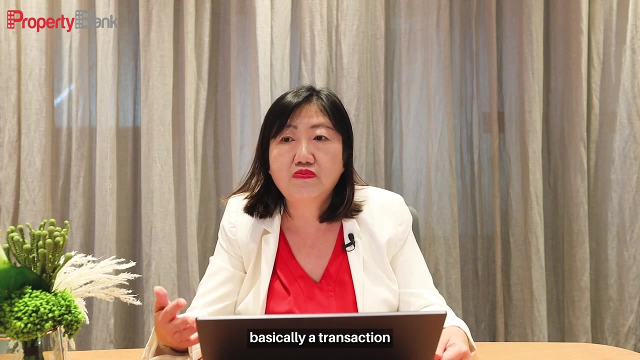 million, quite a sizable deal for, you know, a building of its size, then Parkway Parade. well, the stakes are being held very tightly, but recently there's a 10% interest in the holding stake and that's a basically a transaction of 138 million and equates to about 264 retail shops. 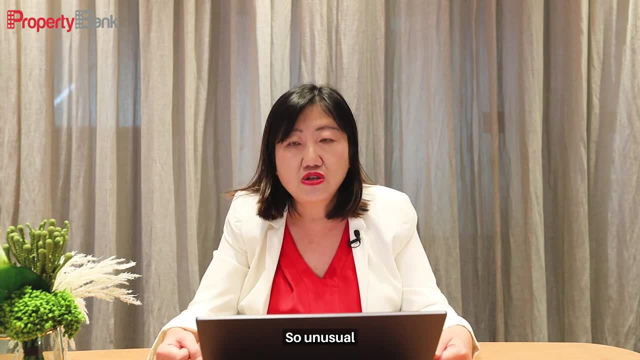 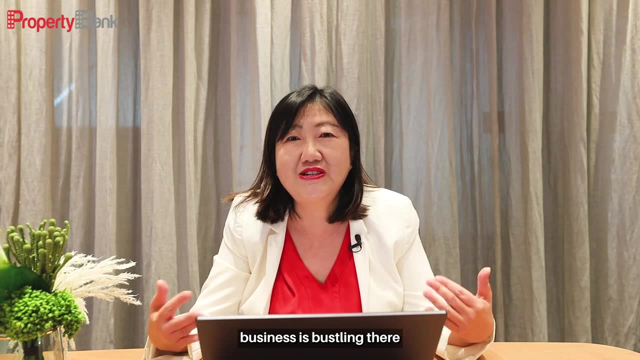 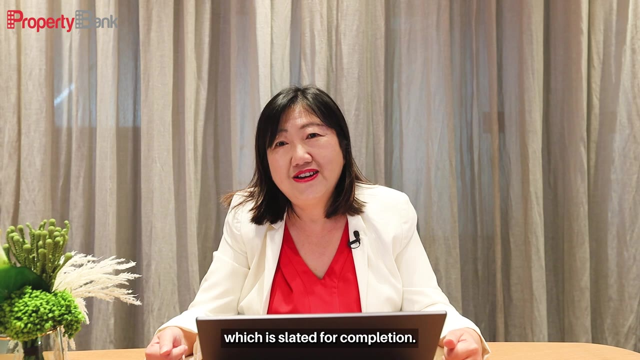 and also 27 strata office units. so unusual, but I would say that Parkway Parade has been known, that you know, business is bustling there and with the upcoming train line which is slated for completion, well, who knows? you know, I mean this guy who had this 10% stake. 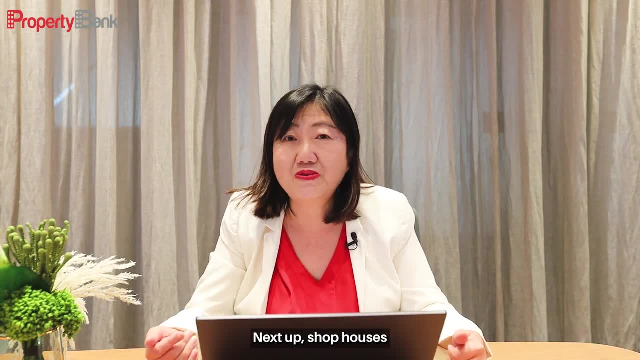 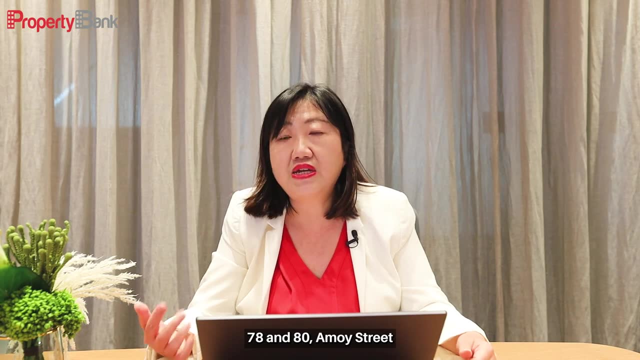 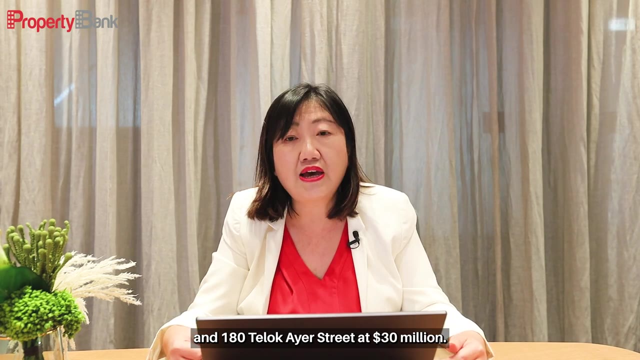 in fact has some foresight. okay, next up shop houses continue to be our darlings. okay, so the sizable shop houses that's been transacted are 78 and 80 Amoy Street at 75 million and 180 Terlo Ayer Street at 30 million. okay, so that's so much. 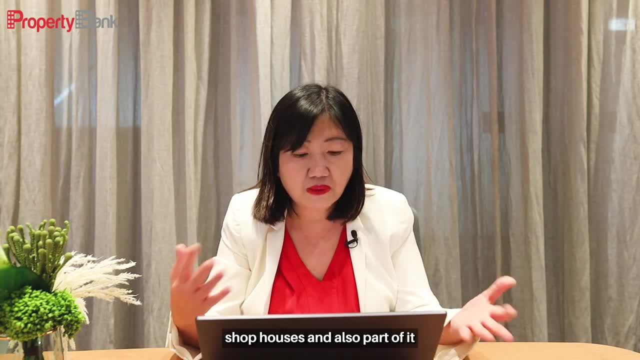 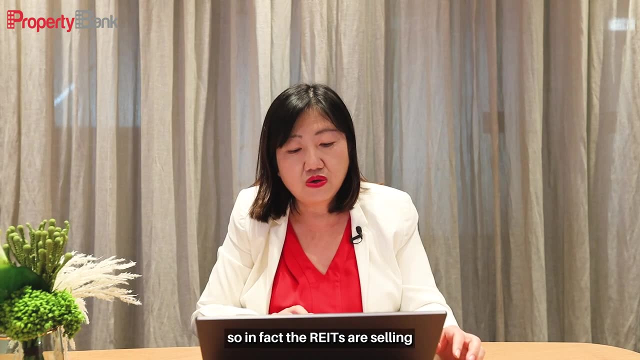 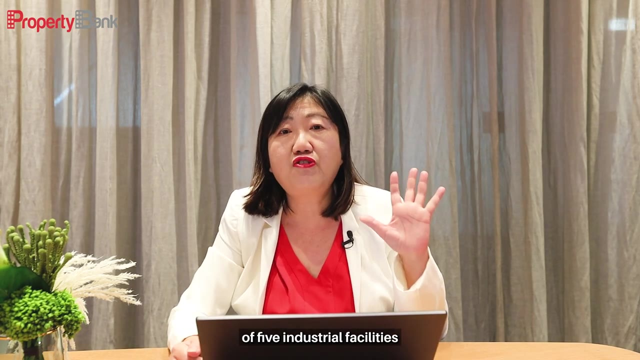 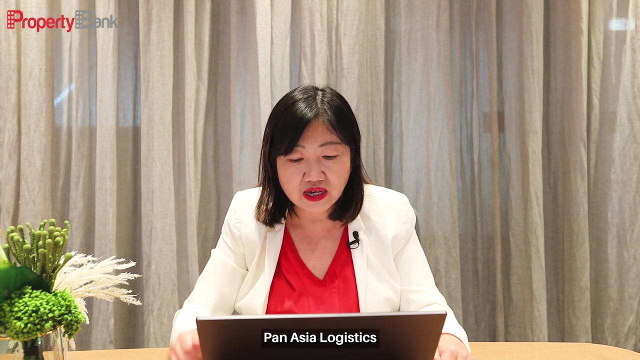 about the office, the, you know shop houses and also part of it, retail. let's come to the industrial, notable contract transaction. so in fact the REIT is selling okay. so ESR has actually sold its portfolio of five industrial facility, which comprises of four and eight Clementine Loop, PanAsia Logistics, Jurong District Centre, 16B Avenue and 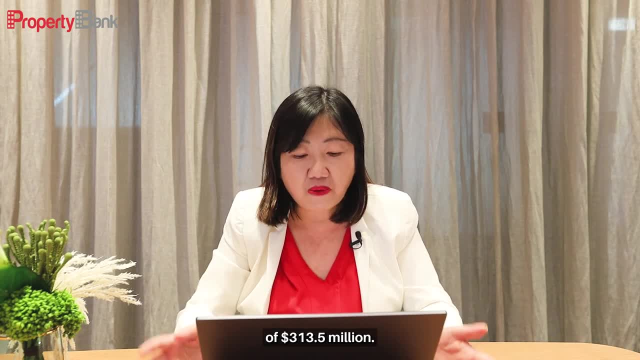 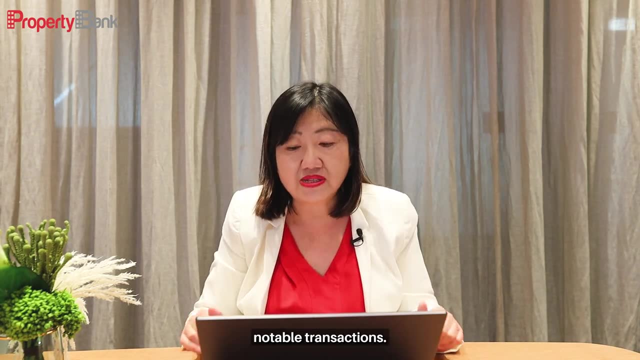 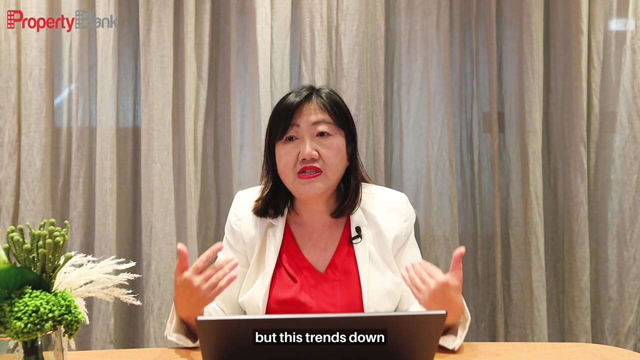 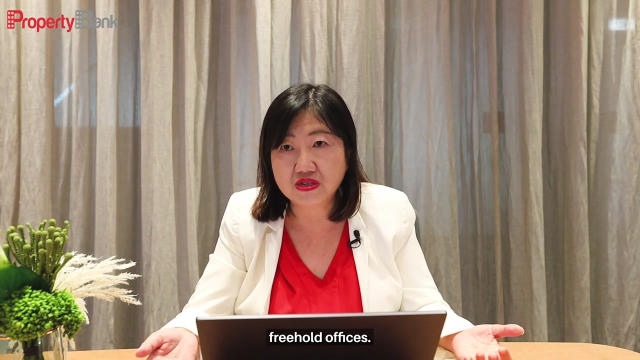 ODC District Centre. so total sum of 313.5 million. so that sums up. you know some of the notable transactions and I think you guys out there, um you, you will not be so much into this, but this trends down to uh, what will continue to trend up, which is basically freehold offices, so freehold. 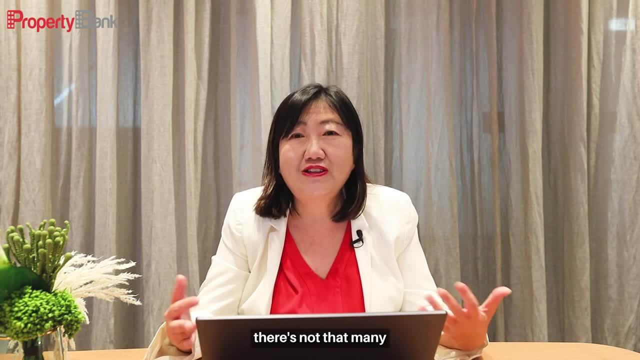 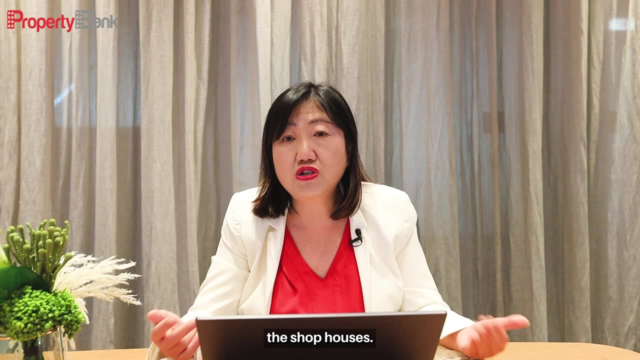 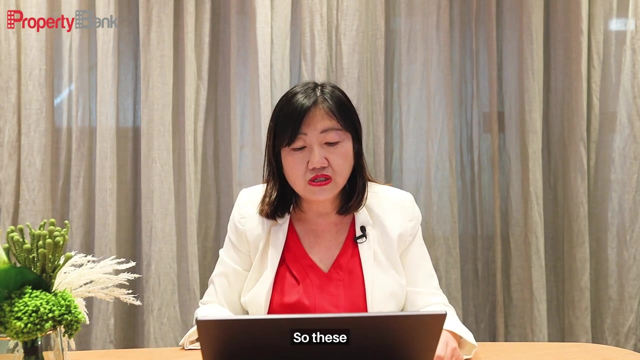 offices. uh, first of all I would say there's not that many in prime CBD, so look out for it. and um then, of course, the shop houses. but shop houses is not everybody's game because the prices have moved up quite a lot. so this, um, companies that bought are institutional. 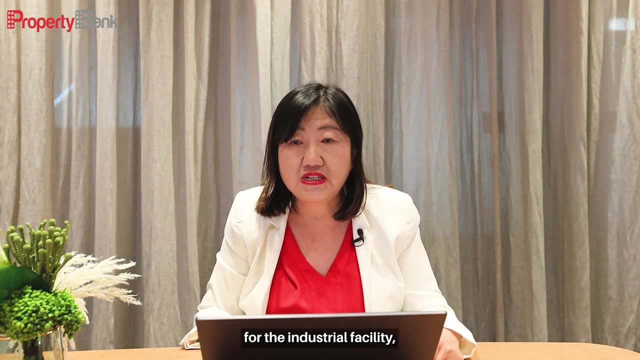 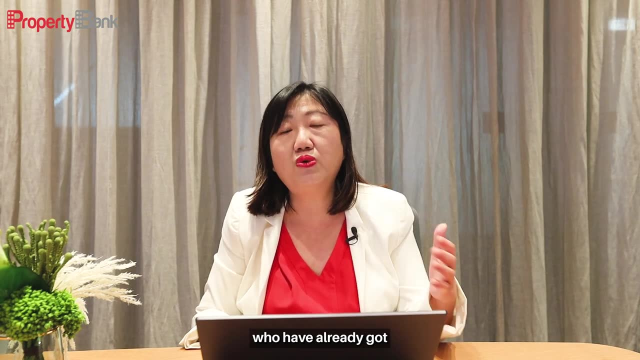 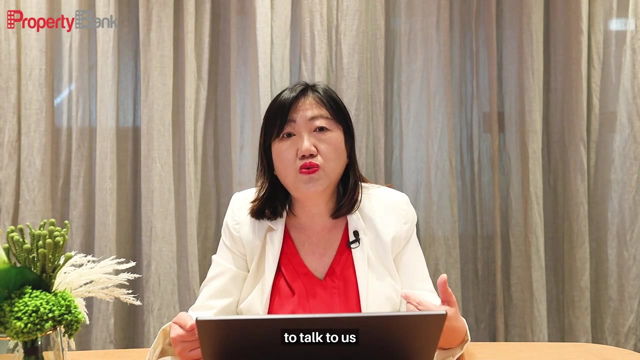 and, of course, for the industrial facility. um, in fact, the trend is right now portfolio purchase. so for those of you who have already got a few sites in Singapore never before, it's a good time for you to talk to us to see how to restructure. uh, maybe you have. 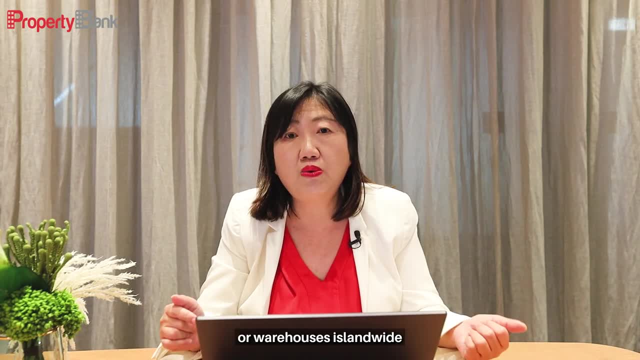 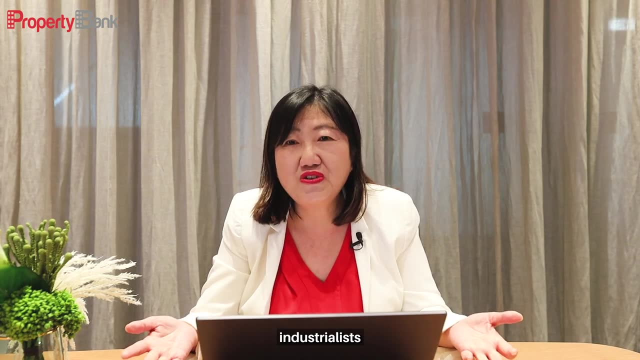 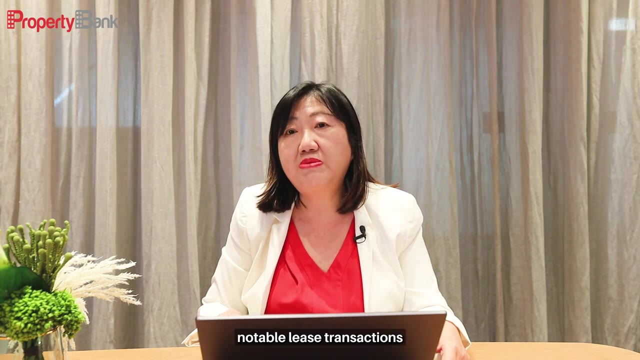 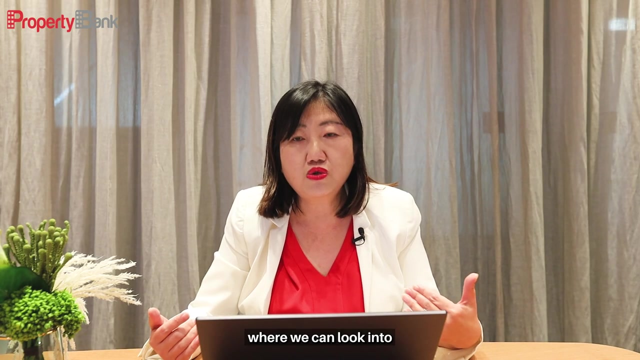 like three to five factories or warehouses Island-wide, so that may be an attraction for the um hungry, uh industrialists who are buying into a slice of the cake, yeah, so next up we want to talk about notable lease transactions, because the rental um is still a big basis where we can look. 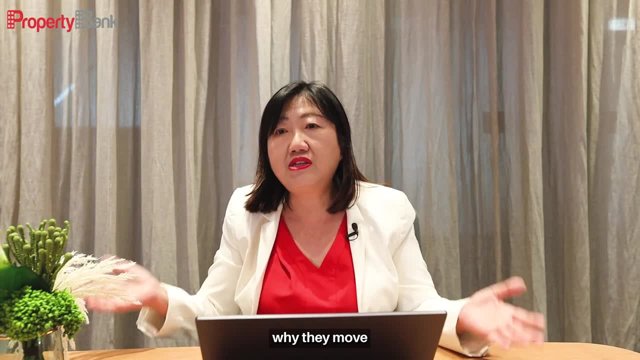 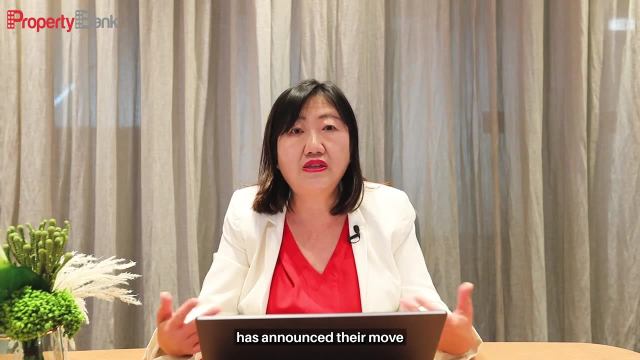 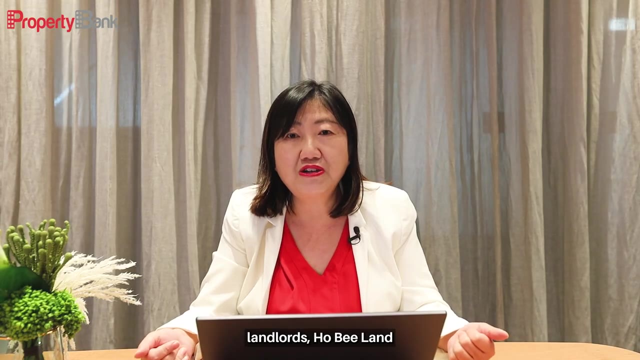 into? uh, who moves from one place to another? why they move? uh, what kind of strategies do they embark upon? so moh has announced their move to elementum, a new building by one of my favorite- uh you know- landlords, Hobie, and a very good location. so they are moving out from. 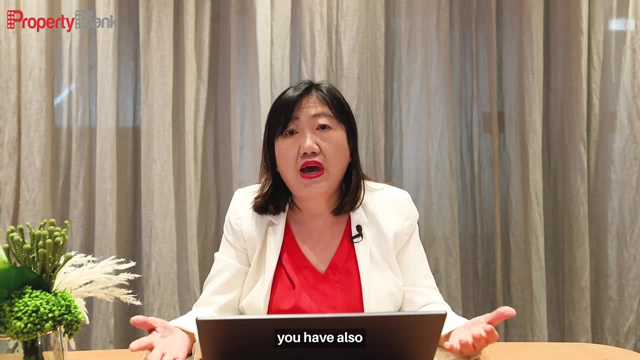 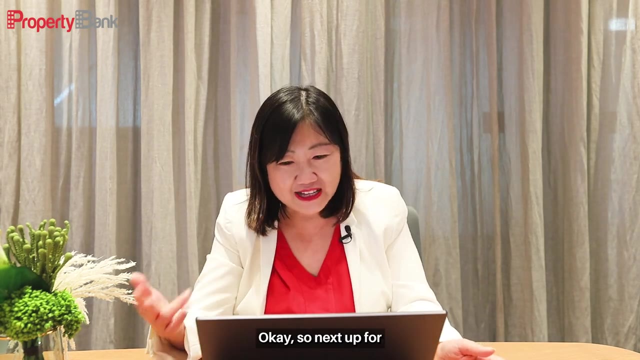 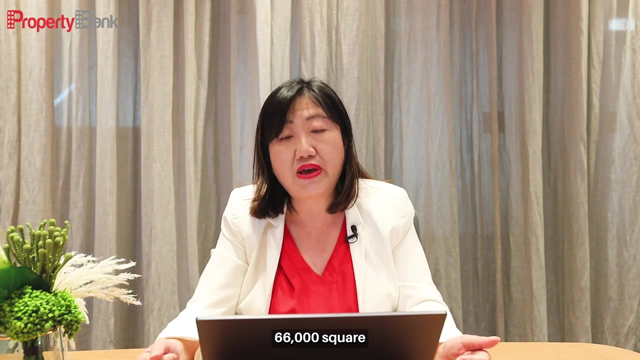 Harper fun Center, and just a few days ago you have also heard about Harbourfront Center having its entrance. out there, you don't know where to move. come to us, okay. so next up for Morgan Stanley, they are relocating 66 000 square feet from Capital Square to ioi Central Boulevard, so that's quite a. 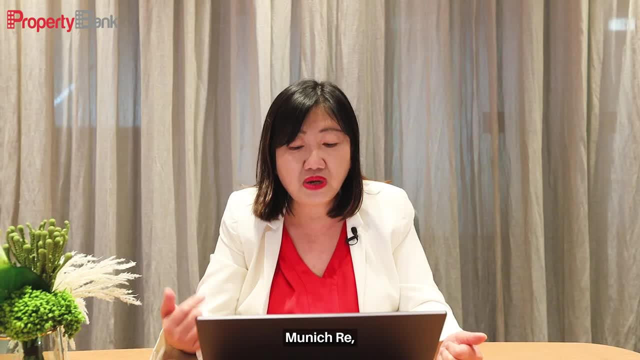 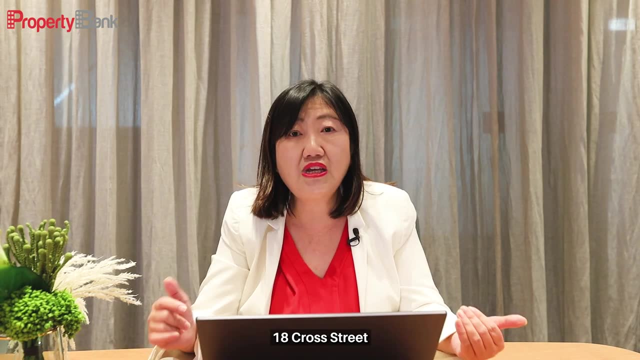 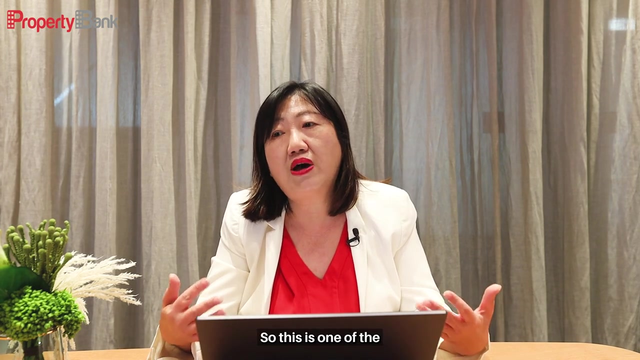 big move as well, and I also like to mention Munich re, which relocates 45 000 square feet from 20 Coyer key to 18 street and 18 cross street, has recently- just um you know- done their refurbishment work. so this is one of the um, i would say: if you don't move to a new building, you move to a building that has. 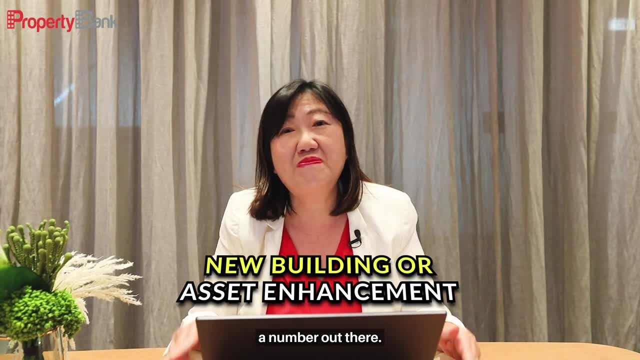 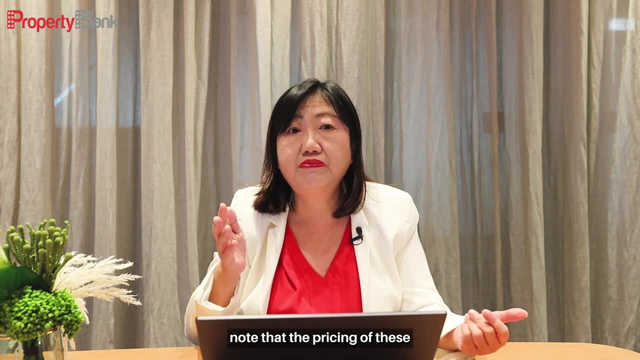 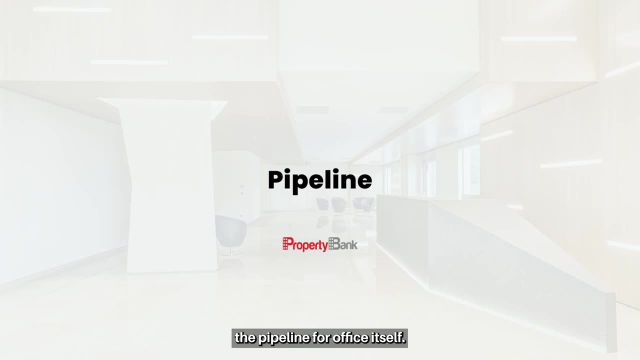 already done some asset enhancement and there are quite a number out there. so, um, it's interesting to, uh, you know, note that the pricing of this um enhanced building is actually much more palatable. so now we look at also the pipeline okay for office itself. um, yes, we know already that ioi. 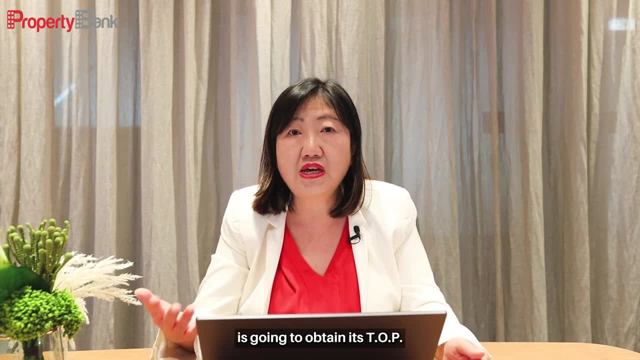 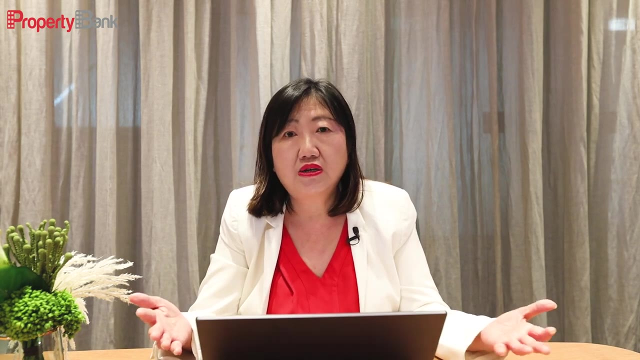 central boulevard towers. um is going to obtain its top third quarter 2023, which is, you know, any time now, um, you know, in a couple of like two, three months, you'll see all some shift and you'll see, um, you know, some vacancy that's in the market. then odian towers extension. 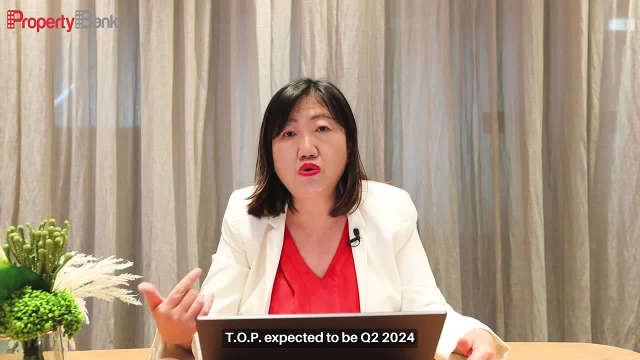 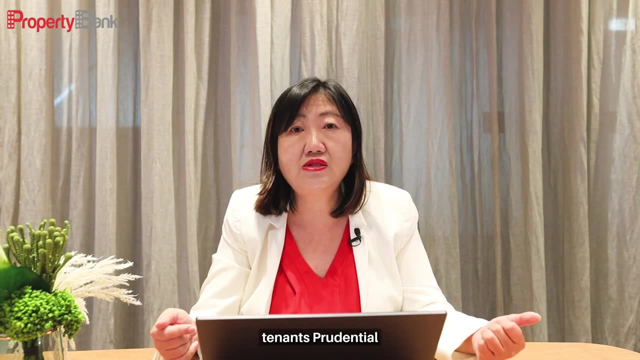 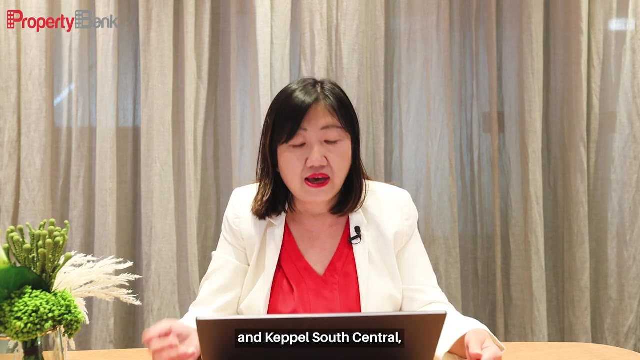 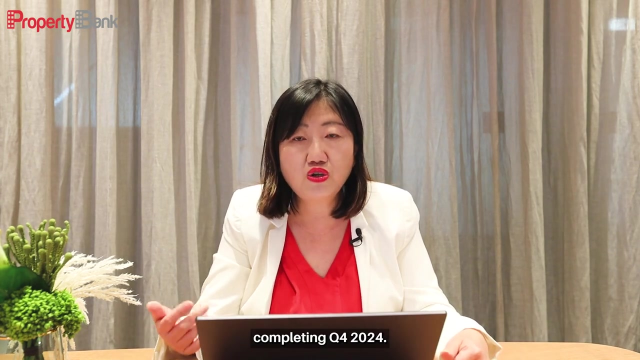 which is top expected to be q22024, labradit towers, which is having one of their anchor tenants, prudential, that will come on stream completing in q32024 and capper south central, which is used to be known as capper towers, completing q42024. so i've actually already sum it up for you between 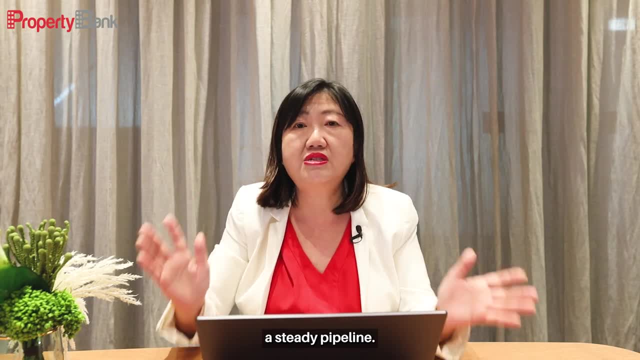 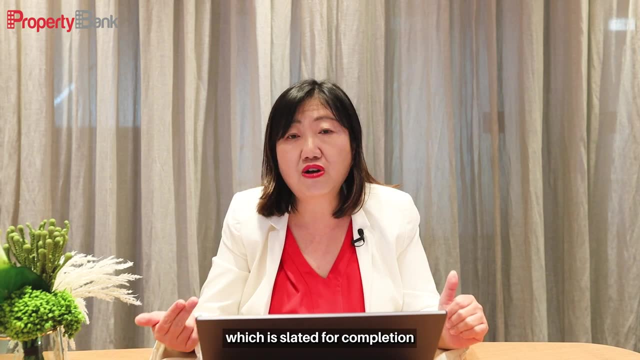 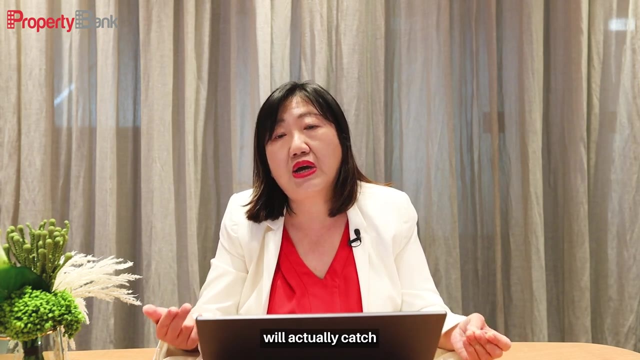 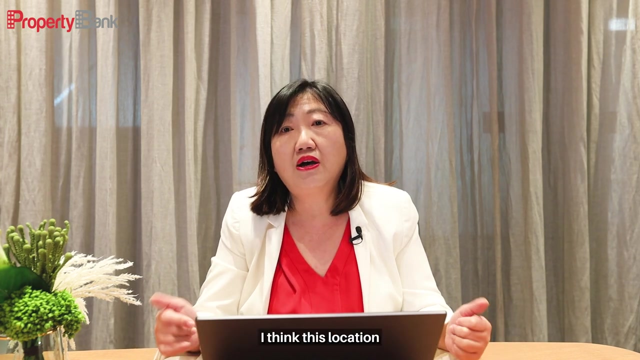 2023 to 2024. so it's quite a steady pipeline and um outside of cbd office, which is, uh, you know, slated for completion in q12025, that's, prior labor green um. so i think that will actually catch a lot of attention because, after the success of plq- prior labor quarters- i think this location 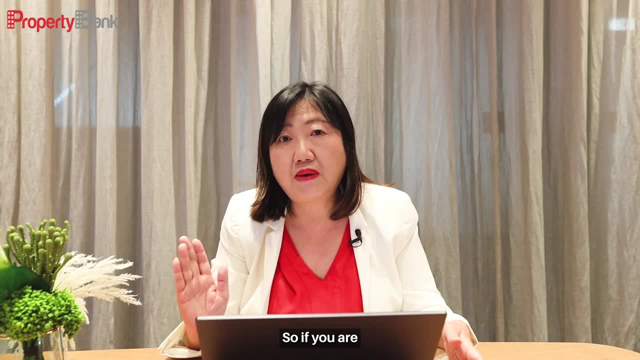 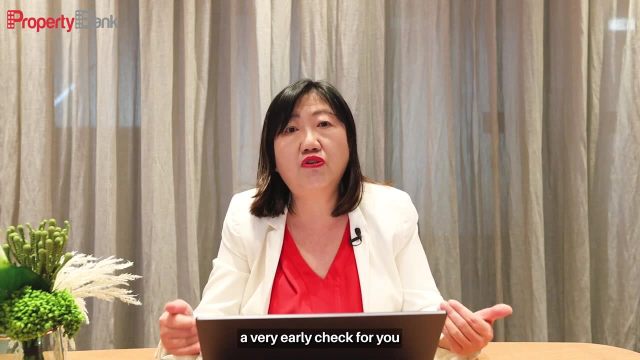 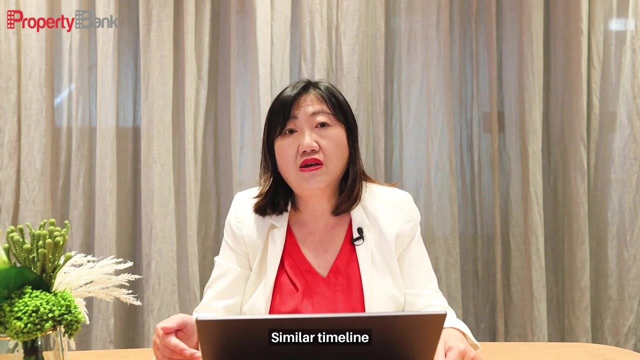 will continue to be attractive. so if you are big tenant looking to shift out of cbd, well we can have a very early check for you so that you can well position yourself into this building. similar timeline, which is outside of raffles place location, is shore tower very actively being marketed right now, also slated for top, expected top. 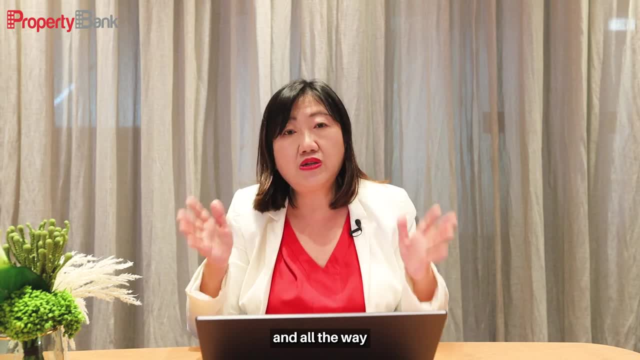 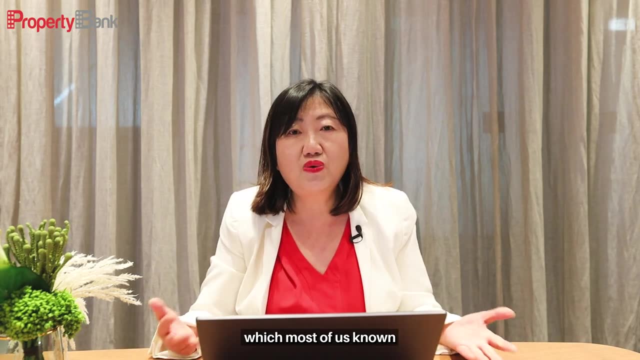 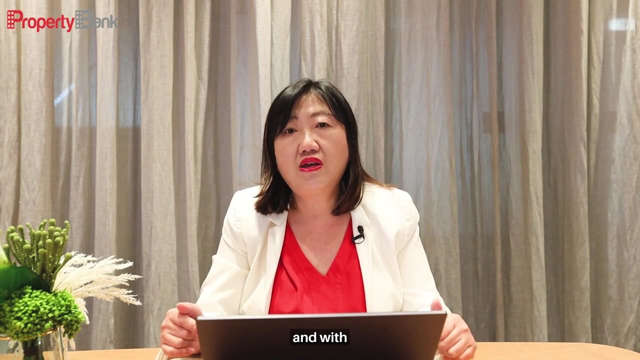 in 2025, quarter one and all the way. we'll also see like for eight, shanton way and even 80 ensign road, which most of us known as fuji, xerox or newport for the residential, the offices will also come on stream 2028. so you can see that for 2024, 2025, there's like a mix of new buildings and 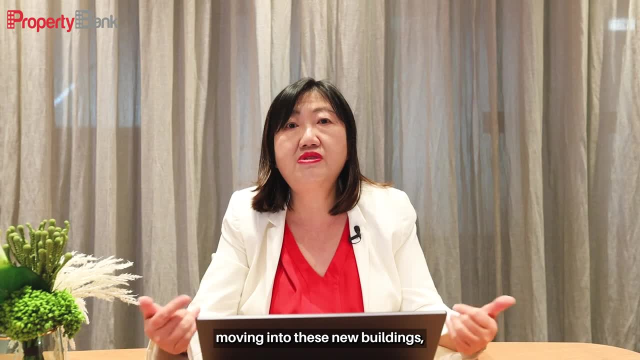 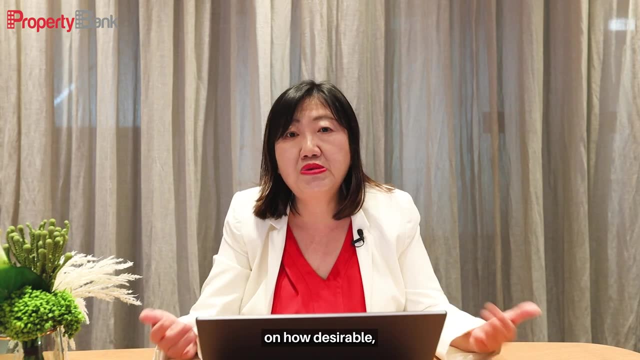 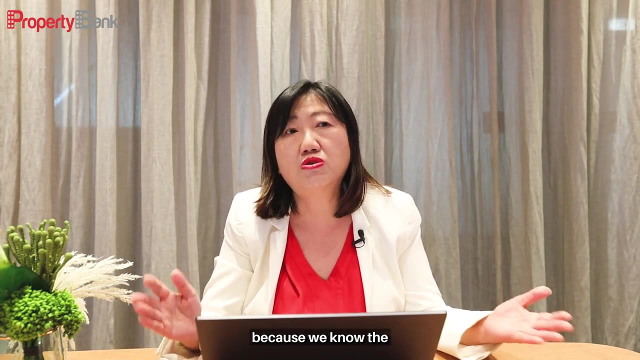 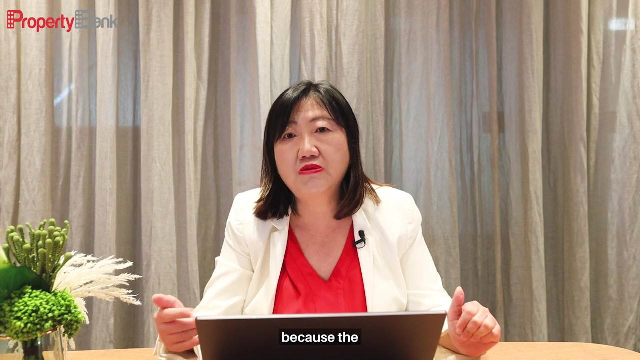 with companies moving into these new buildings, so you can also have a chance to take over the fully fitted condition, depending on how desirable, how matching to your- uh, you know- space. i think we are ready anytime to talk to you guys, because we know the movers of the market, where they are going to move to and, um, you know, take, take some time. 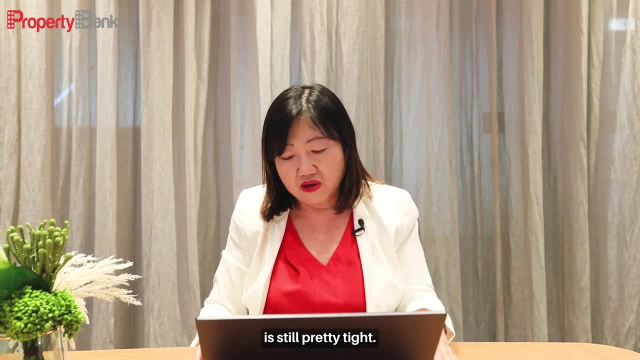 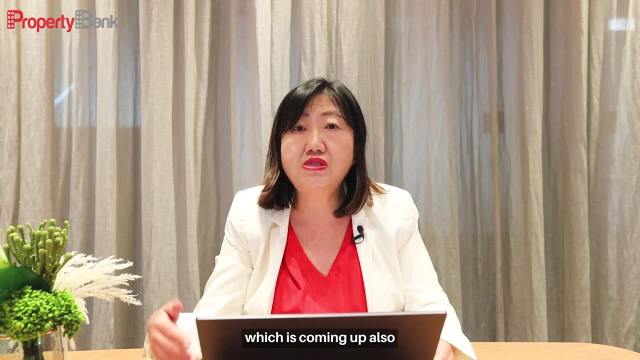 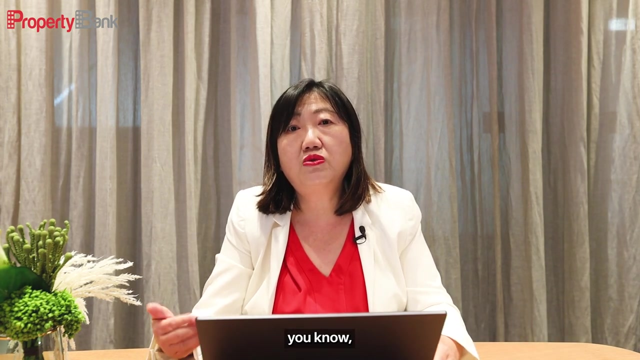 because the the supply of office is still pretty tight. okay for industrial, of course. we know that um, there's this, uh pongo district, uh you know, which is coming up also, uh, with the university moving there, and i think, um you know, the the first few tenants already inked their deal over there. it also can be an interesting location. 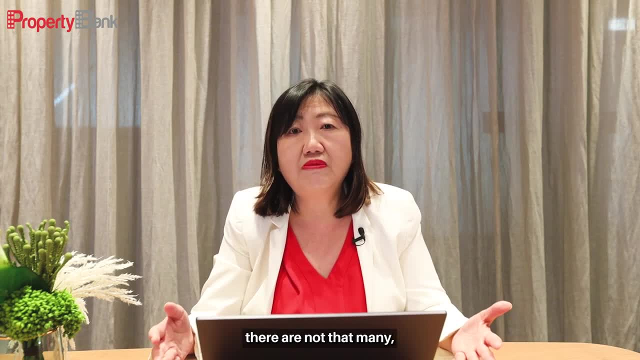 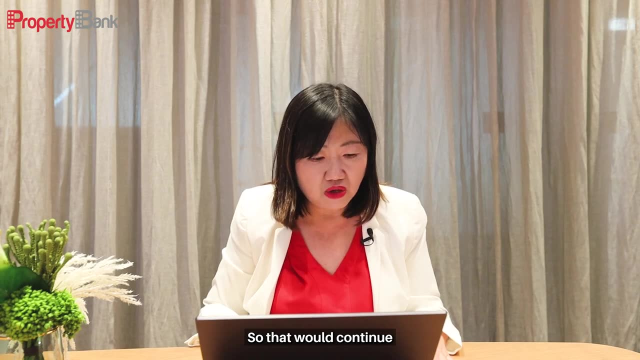 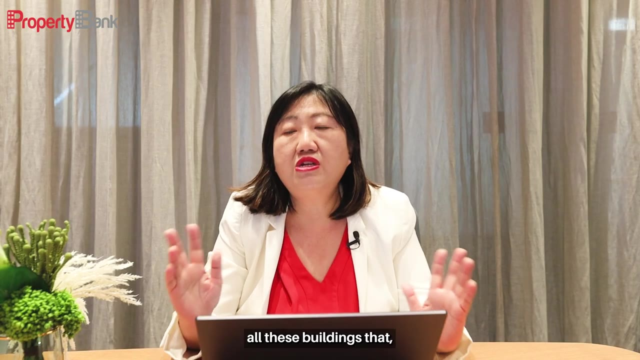 because in the northeast location there are not that many, i would say, high-tech kind of space for the industrialists. so that would be continue to be interesting. so, to sum up, so how about the new buildings that you guys are moving to? um, the new buildings are a lot, you, you realize that. 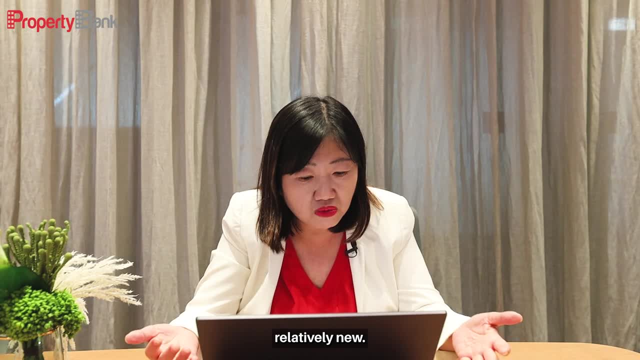 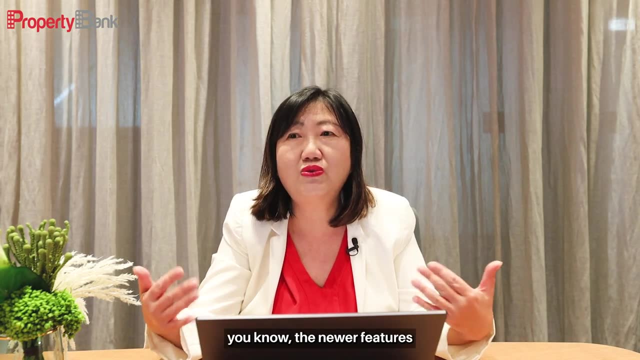 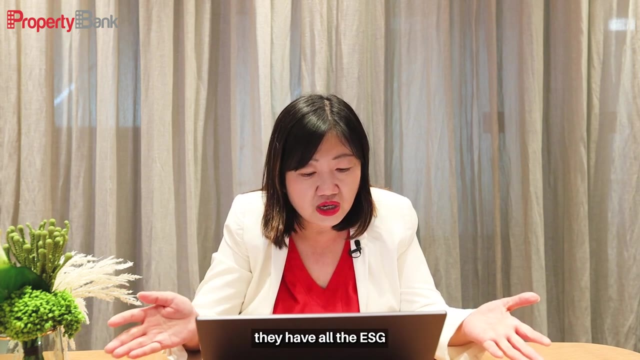 all these buildings that, um, you know, companies, big corporations, move to, uh, buildings. that's relatively new. so why do they move to these spaces? is because of, of course, you know, the newer features and i think these new buildings are definitely green mark. they have all the esg initiatives in place. 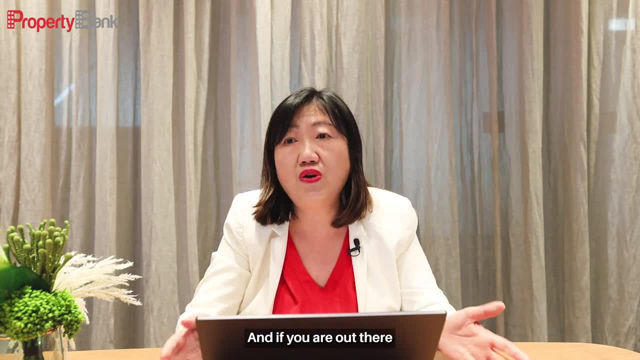 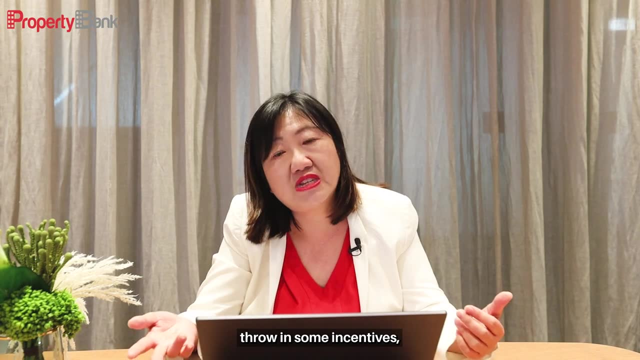 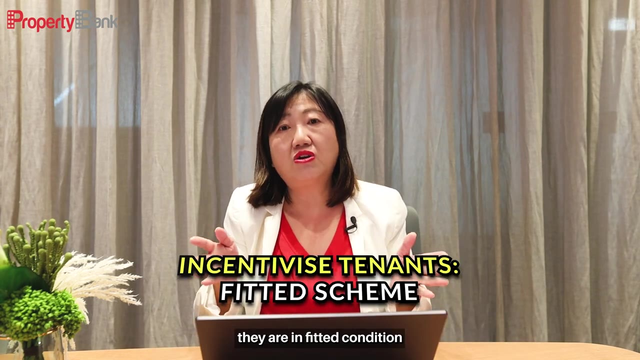 a premium to move on to all these new buildings. and if you are out there as a landlord and you are in the so-called slightly older buildings, throw in some incentives. perhaps you can even talk to us. we can plan your space such that you know they are in fitted condition so that your 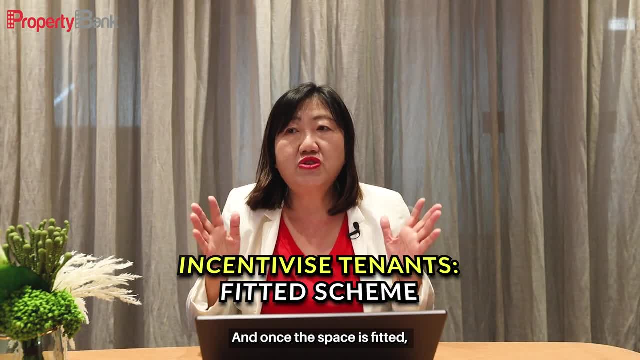 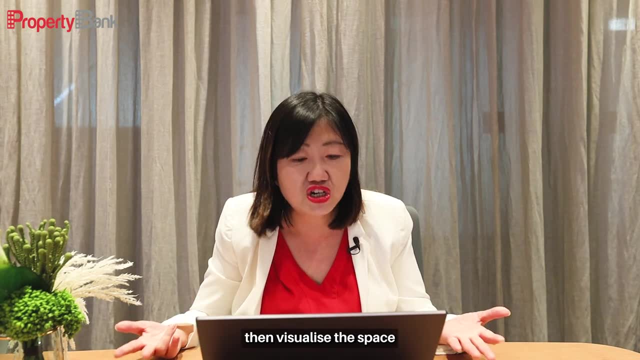 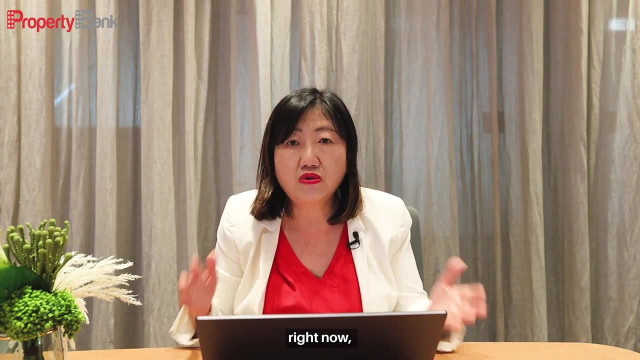 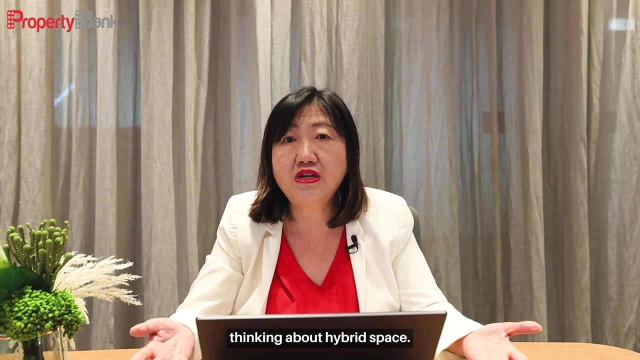 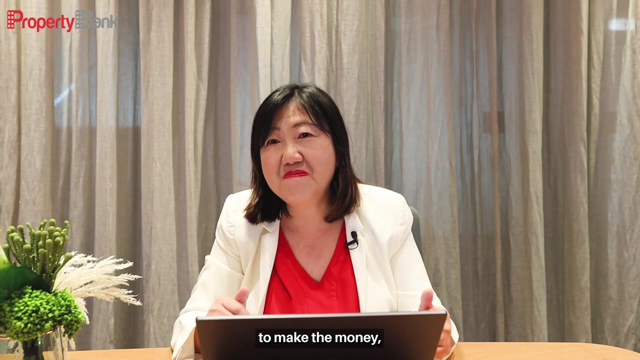 tenants can save some fitting out and once the space is fitted, the way to sell is much easier because the tenants can then visualize the space and, of course, for landlords- right now they, you guys- should also observe that there is um likelihood of thinking about hybrid space. so instead of um, you know, getting your co-working tenants to make the money, 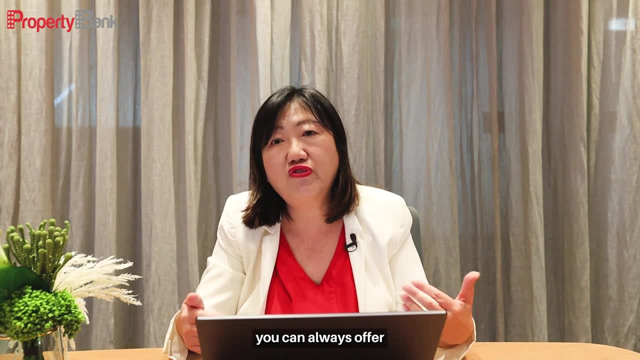 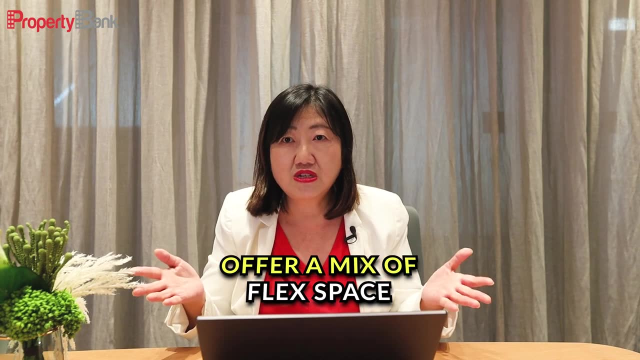 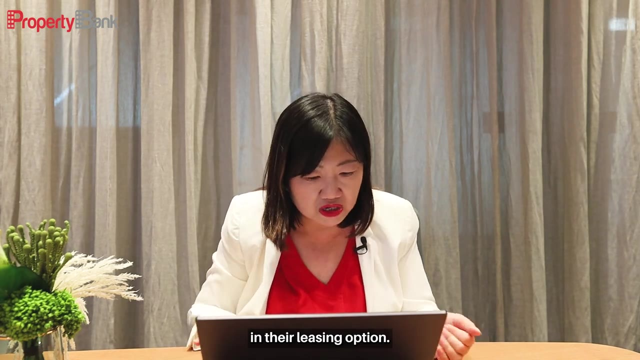 some of you out there. as landlords, you can always offer the call, which is the conventional office, and a mix of the flex space, where the tenants can take shorter period or can just, you know, be more flexible in their leasing option. yeah, so now next up, which is you, the tenants. 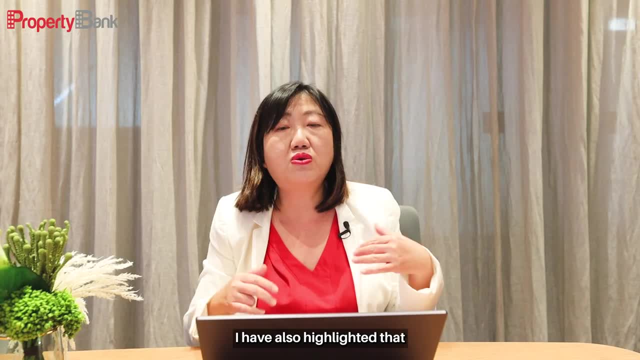 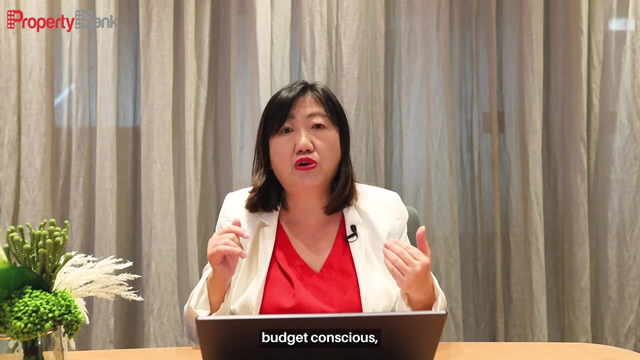 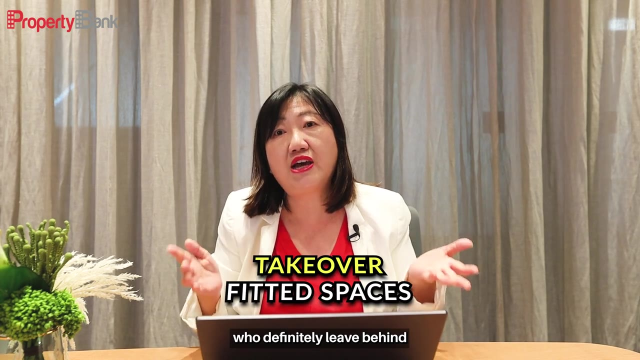 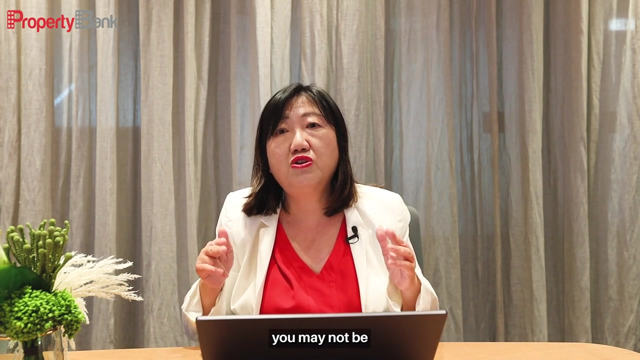 okay. so in fact, uh, like earlier, i have also highlighted that, with all these major tenants moving into new buildings, and if you are budget conscious, you can take over some of the fittings from, uh, these corporate tenants who definitely leave behind very good fittings. so what you lack is probably, you know, the time to plan. of course, you may not be so readily. 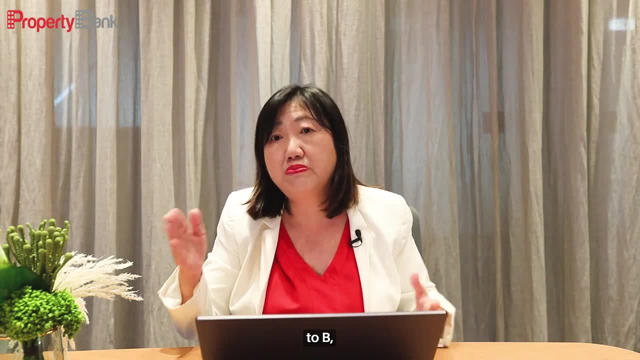 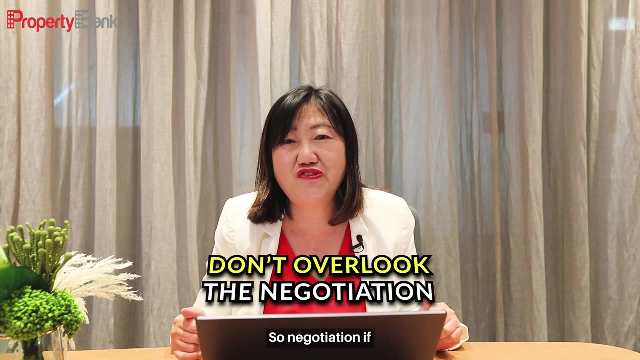 understanding or knowing who is going to move from a to b and um, i think nothing beats about the negotiation. so negotiation, if you directly go and find the landlords and you think you can do the best job, landlords know they can do the best job. they can do the best job. they can do the best job. 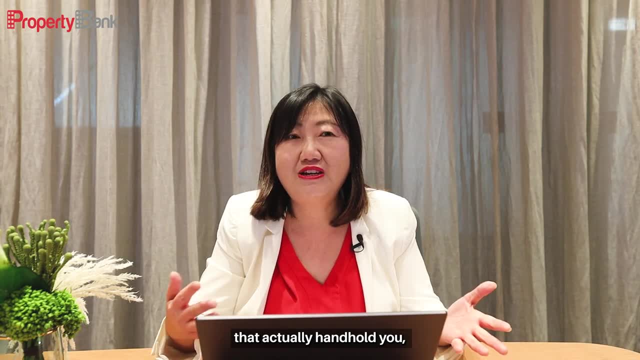 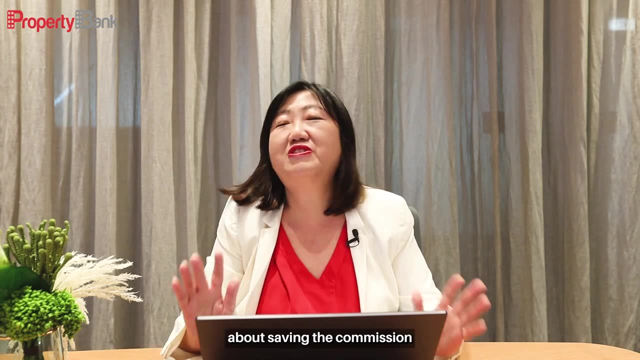 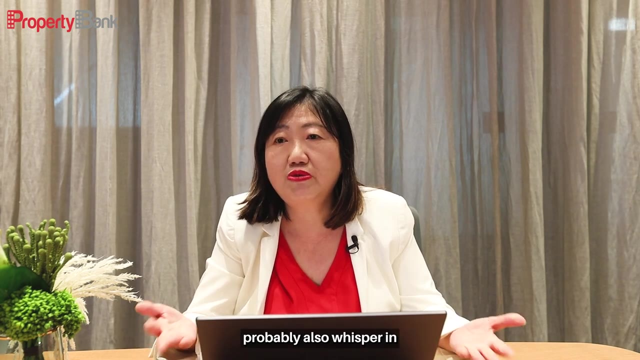 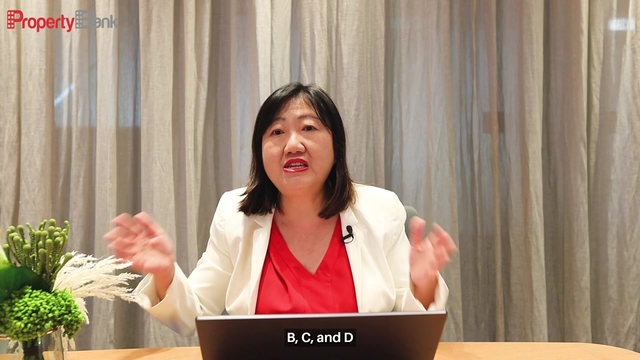 that you don't have someone that actually handhold you. in fact, the contrary is. the truth is that landlord is not too bothered about saving the commission with advisors helping you, but advisors would then probably also whisper into landlord's ears. you know this particular tenant is looking at a, b, c and d and encourage landlords to be more competitive in their offerings to you. 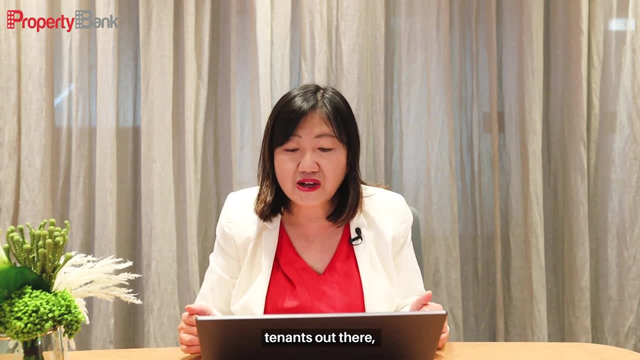 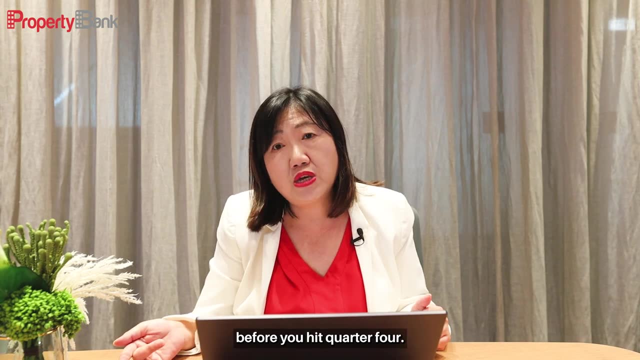 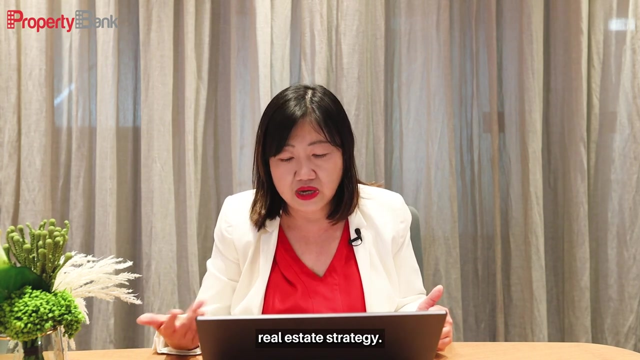 so, um, yeah, uh, occupiers out there, tenants out there, yeah, this is uh one good time that you uh, because now you're into quarter three, before you hit quarter four. um, it's a good time for you to sit and rethink your real estate strategy. and earlier on, where we actually highlighted the 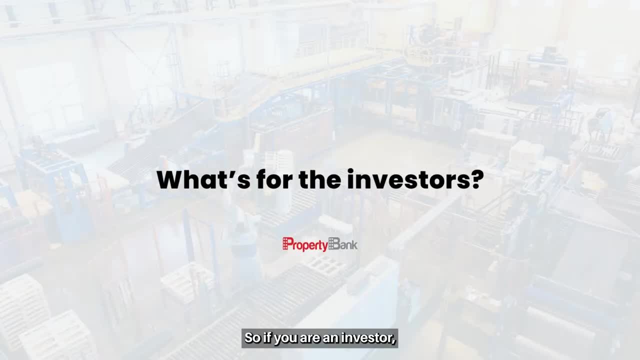 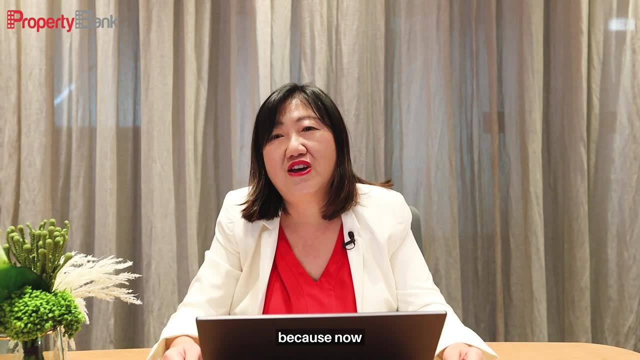 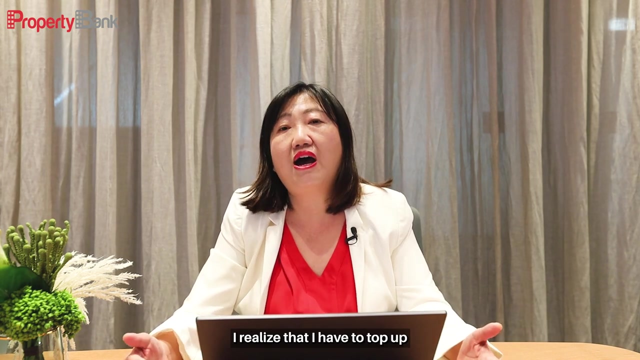 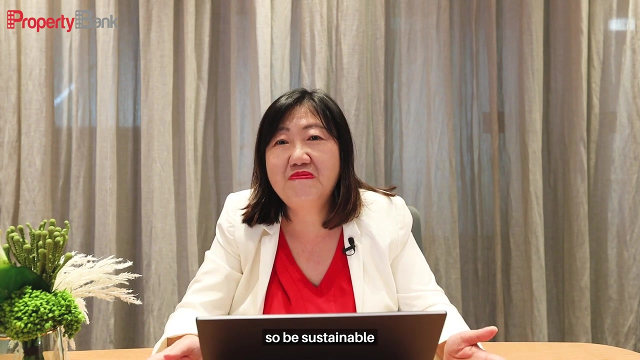 notable sale transactions. so, if you are an investor, what are you actually going to look at? well, i would say long term, because now we are at an all-time high for your interest rates and, in fact, me, as an investor, i realized that i have to top up my monthly installment. so, uh, be sustainable in your financial planning, because, uh, for now,